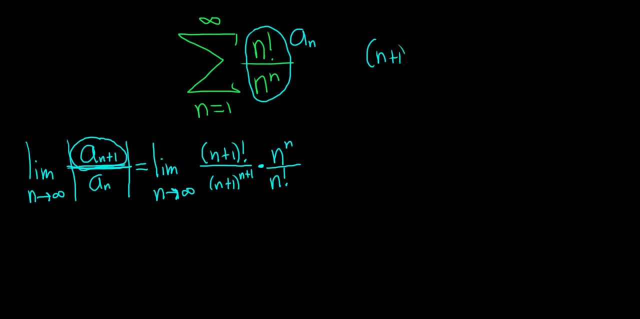 First notice: if you have n plus 1 factorial over n factorial, Well, n plus 1 factorial is n plus 1.. And then you subtract 1. Then it's n n minus 1, n minus 2,, et cetera. 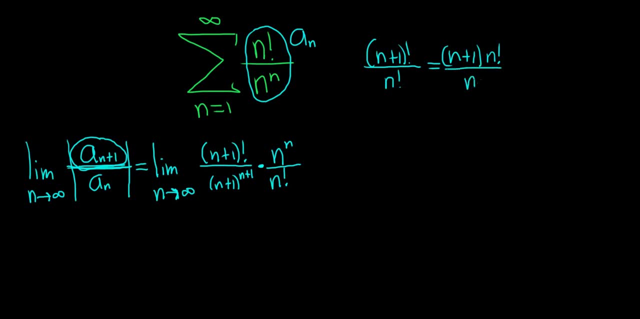 So the rest of it is simply n factorial. So these cancel and you're left with n plus 1.. So this is equal to the limit as n approaches infinity. So we have n plus 1.. Then we have n to the n over n, plus 1 to the n plus 1.. 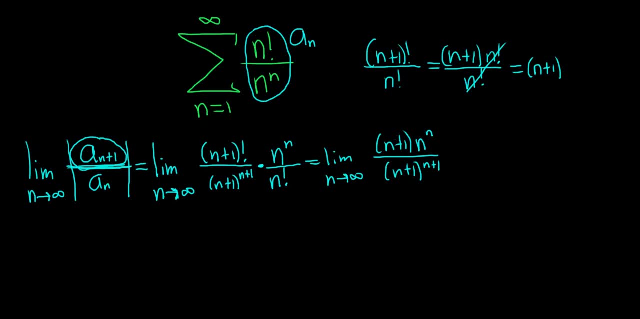 Ah, I see something else That can. That can simplify now. So this n plus 1 is being divided by n plus 1 to the n plus 1.. So we have n plus 1 to the n plus 1.. So check this out. 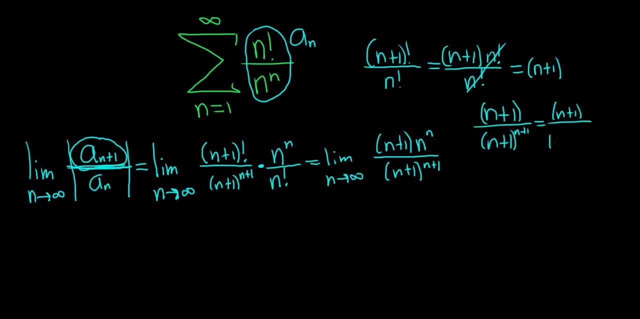 This is n plus 1.. And then this is n plus 1 to the n times n plus 1 to the 1, right, Because when you multiply these you actually add the exponents. This is really nice. This is 1 over n plus 1 to the n. 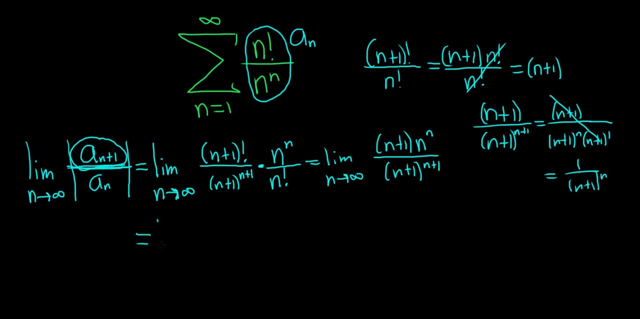 So let's go ahead and make that step next. So this is equal to the limit as n approaches infinity. So we still have the n to the n upstairs, And on the bottom we're left with n plus 1 to the n. 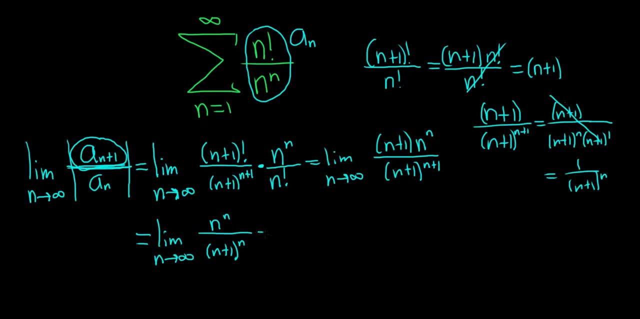 So what could we possibly do next? Well, I guess everything is to the nth power. So let's try to do that: Raise everything to the nth power, Because we have n to the n over n plus 1 to the n, That's really n over n plus 1 to the n. 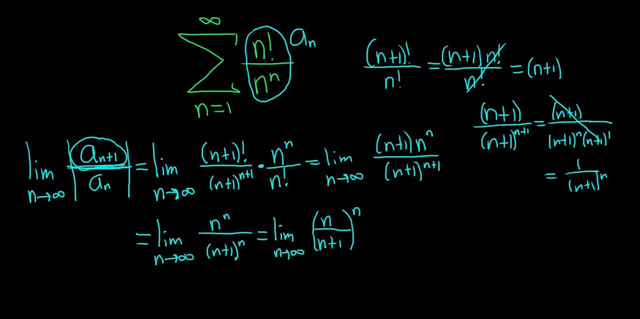 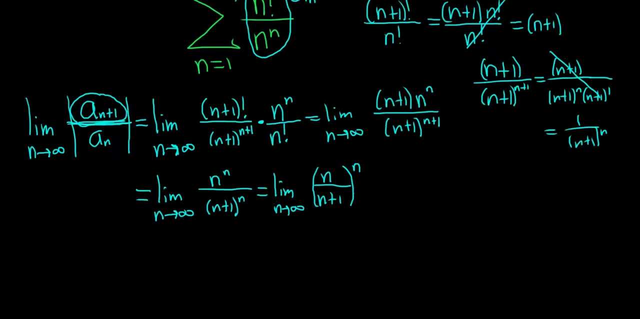 And this should remind you kind of of something. maybe. If it doesn't, let me show you. You see, I've done this problem before. It's been a long time, But I know there's a trick. And here is the trick. 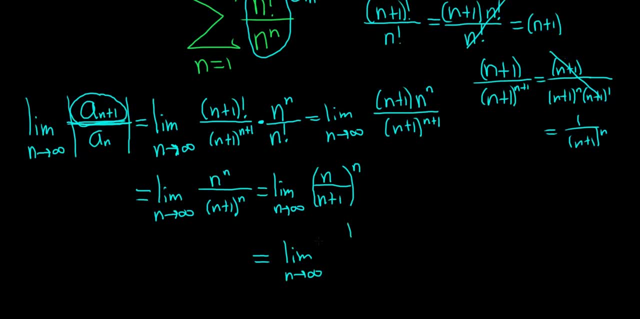 The trick is, you want to write it as follows: This is really 1 over n plus 1 over n. Pretty sure this is the trick. We're going to find out. We're going to find out if this works. You say what just happened?